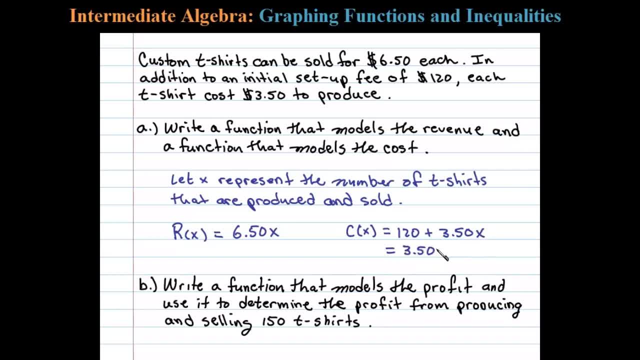 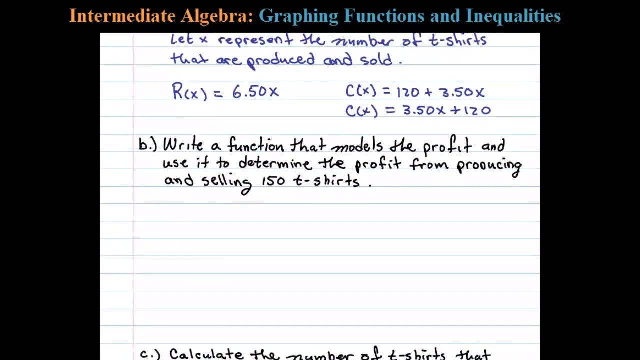 Let's write this as 3.50x plus 120.. That's our cost function. Now we'll use these two functions to determine a profit function. Here we not only want to determine a profit function, we want to use it to determine the profit from producing and selling 150 t-shirts. 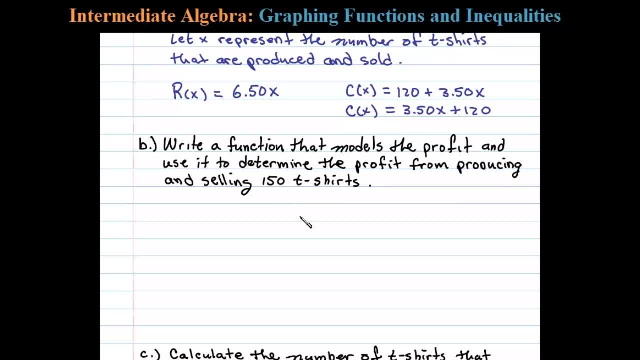 Now, profit is equal to revenue less costs. In other words, P is equal to our revenue, R minus our cost, C. In this case the revenue is 6.50x minus the cost function here, 3.50x plus 120.. 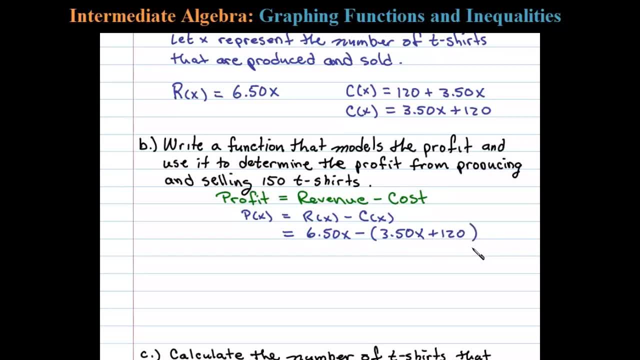 Notice. I took care to put this cost function in a parenthesis to remind myself that I have to apply the distributive property And that gives us 6.50x minus 120.. So we have 3.50x minus 3.50x minus 120, which equals 3x minus 120. 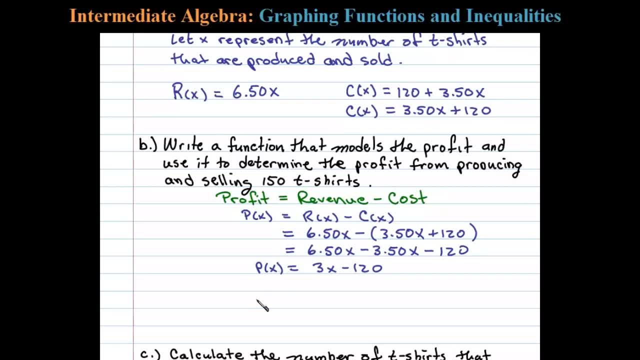 This is our profit function. Now we're going to use this to determine the profit of producing and selling 150 t-shirts. So we substitute 3 times 150 minus 120.. In this case we get 4.50x minus 120, which equals $330. 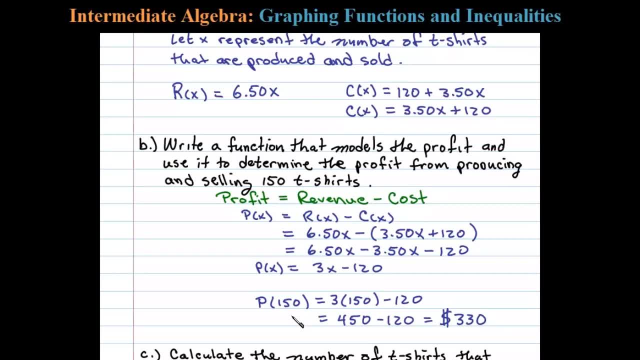 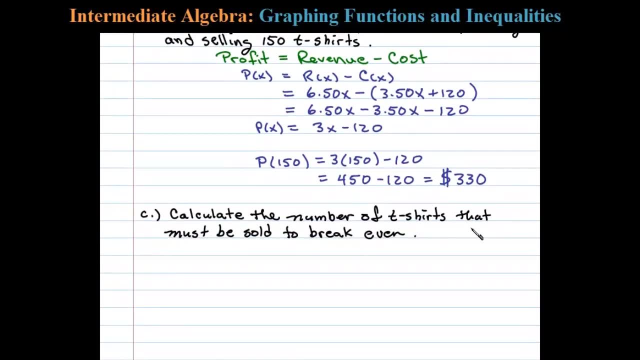 That's our profit from producing and selling 150 units. Next, we're asked to calculate the number of t-shirts that must be sold to break even. Now, to break even, profit is equal to 0.. And in this case, we found that our profit function was equal to 3x minus 120..